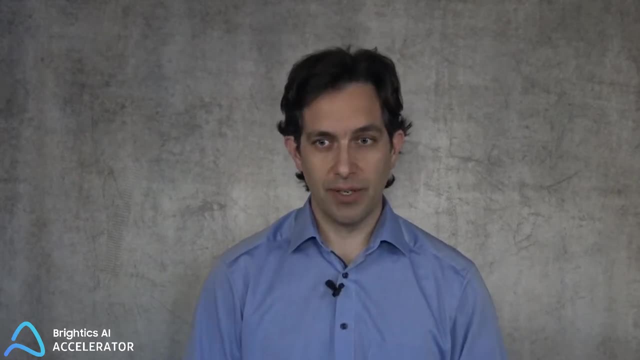 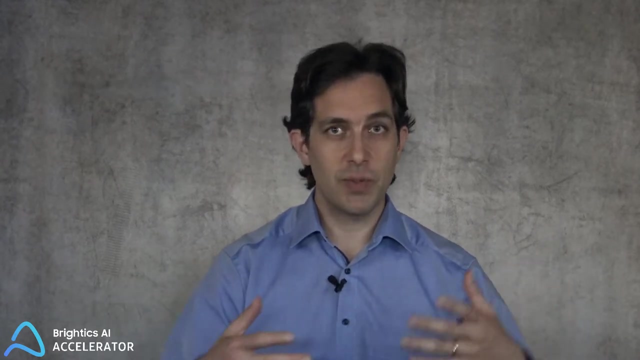 And in trial and error or trying many varieties and simply choosing the best, we have to remember the most important question of all: How do we define best, How do we compare two possibilities? Which one is better out of these two possibilities? You know this in life, right. 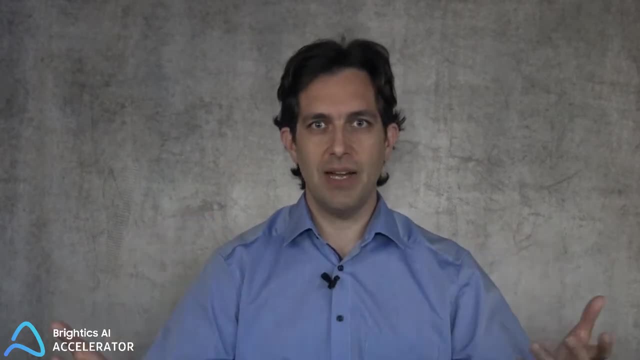 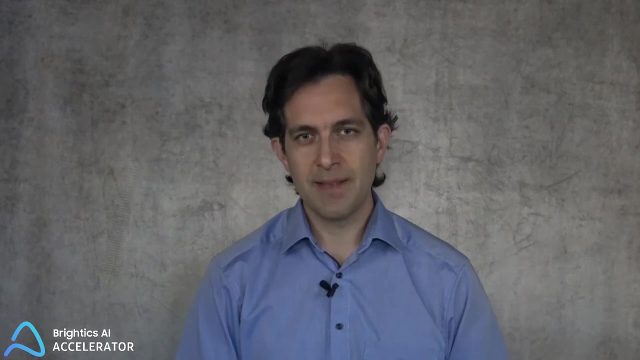 You're trying to buy a house. Which one is the best house? It's not necessarily the cheapest or the biggest or the prettiest or the one with the best school district. It's a combination of all of these things. The same thing applies in machine learning. 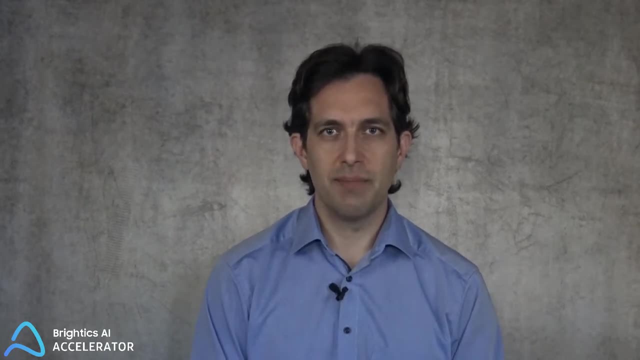 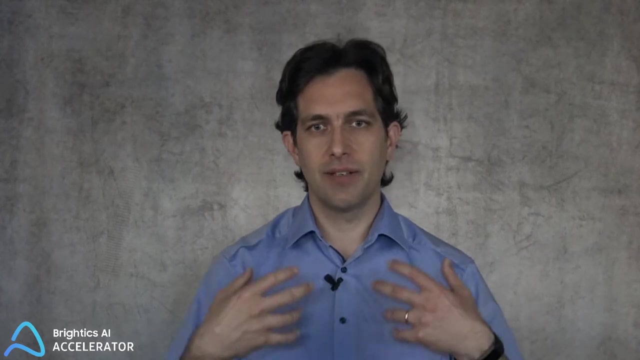 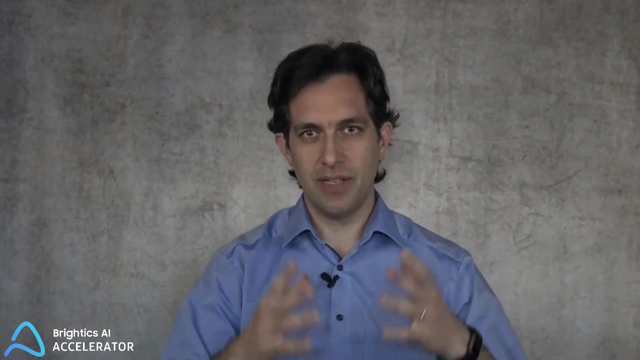 We have to define what we mean by best. Now, there are three major criteria that go into this. They are accuracy, Precision And model complexity. Now let me just illustrate what I mean by that. Let's suppose we're playing darts. 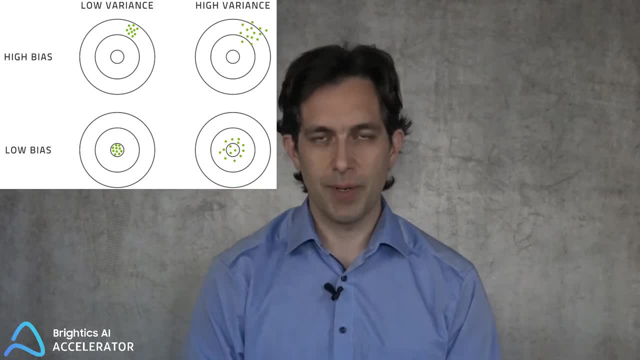 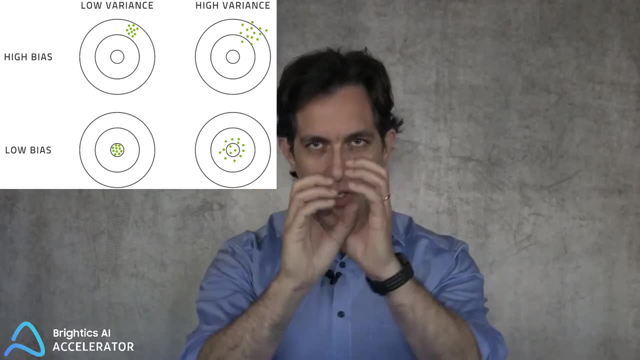 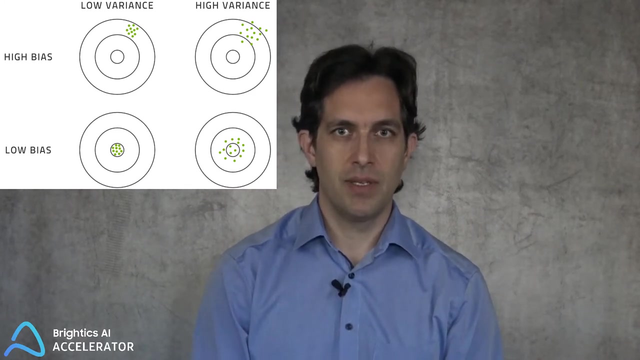 So I'm taking a dart and I'm throwing it at the dart board. I repeat that several times. If my darts are closely collected with each other, that means that they have a small variance Right. That means the precision of my model is very high. 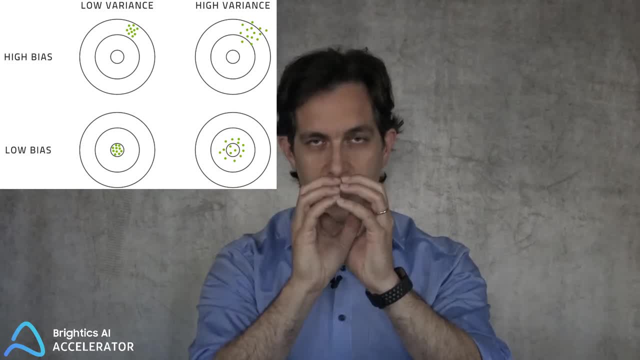 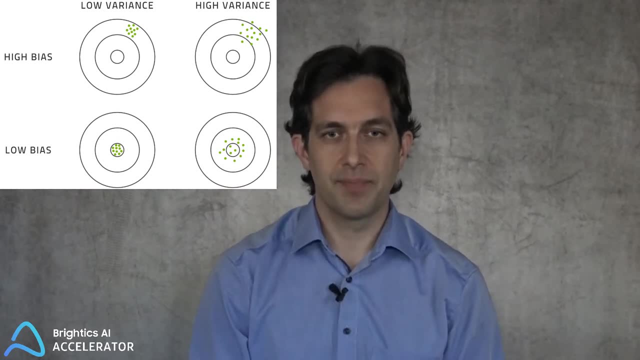 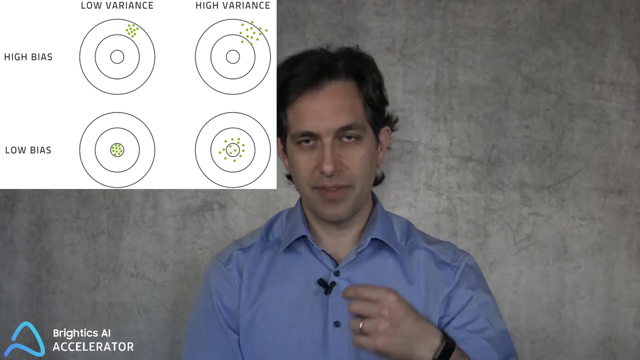 Now, if that tight cluster of darts is right at the center of the dart board, that means that I have high accuracy, Right? This is referred to as low bias, Right, If I'm very accurate, if the result of my algorithm is correct, then I have low bias. 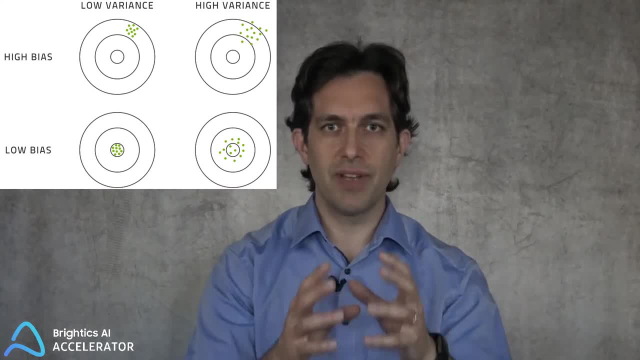 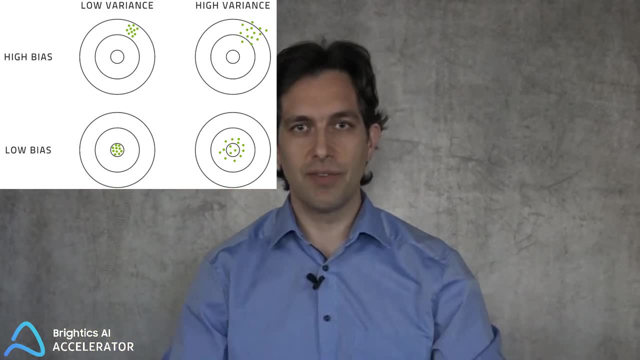 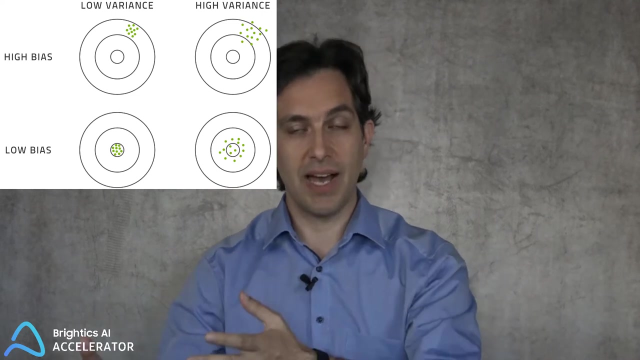 And if I have very little scattering then I have low variance. But I can have low variance off-center somewhere. Then I have high bias, low variance. I can have a great deal of scatter but on average- be right, that would mean I have low bias but high variance. 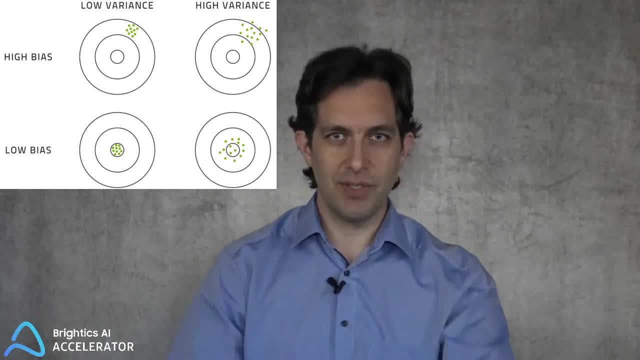 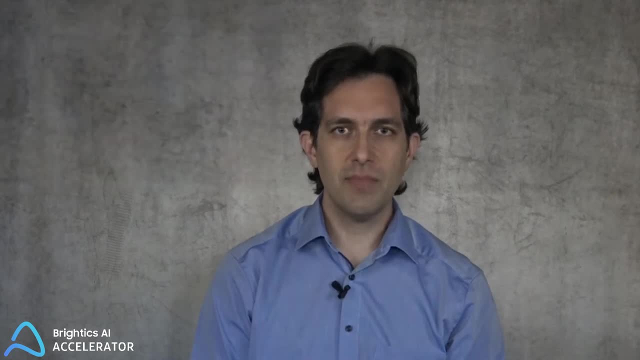 And, of course, the worst possibility of all- I can be scattered off-center Right, In which case I have high variance and high bias. Of course, what I want is to have low bias and to have low variance. I want to be accurate and precise at the same time. 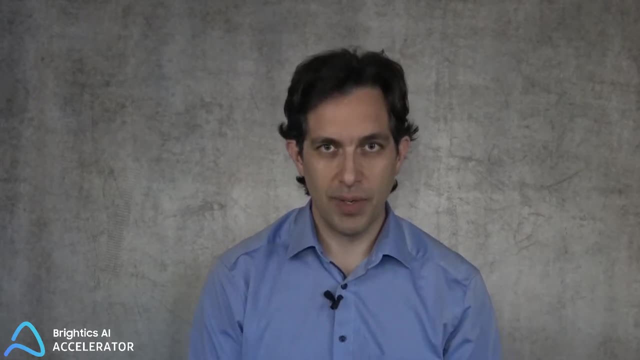 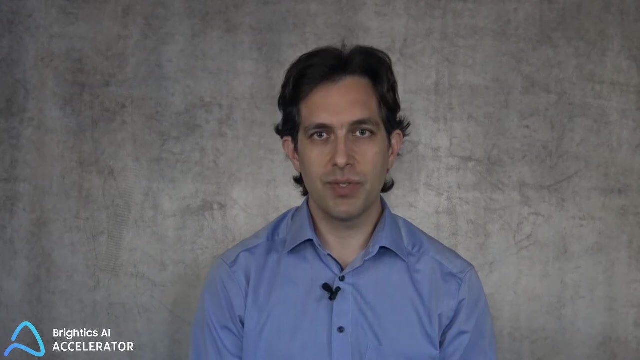 Now the third component here is model complexity. With a very simple model I'm going to underfit. The model will be too simple to encompass the complexities that are present in my data set. As the model gets more and more complex, it will be able to represent the dynamics in my data set. 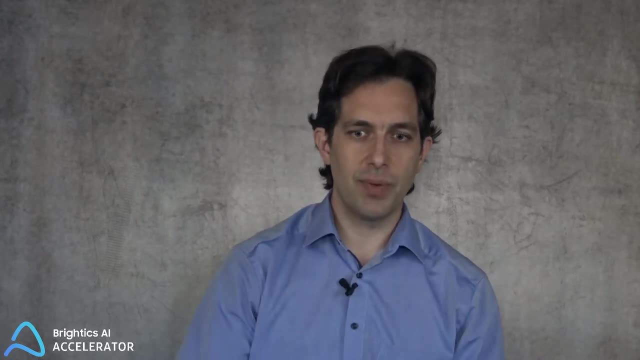 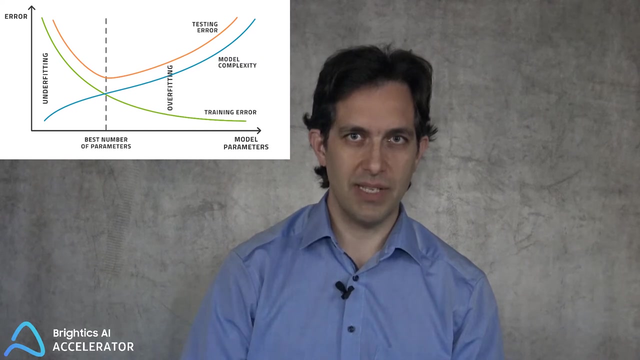 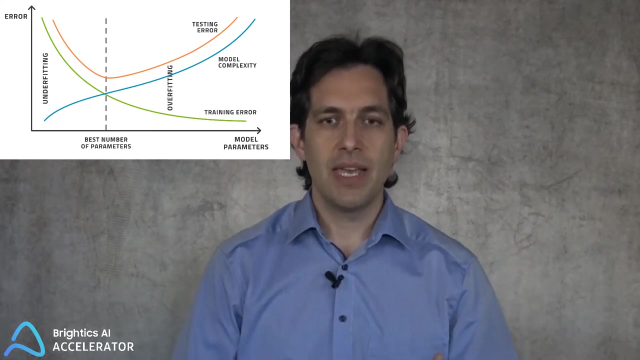 Eventually it will reach a certain level of complexity, And when it reaches the point where the model becomes so complex, it will be able to kind of memorize the contents of the data set and no longer learn the underlying dynamics of what makes this data set the way it is. 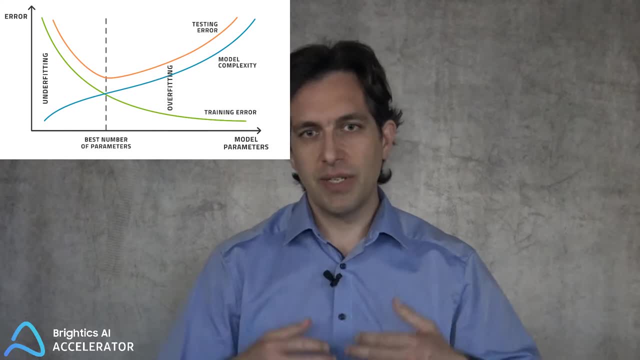 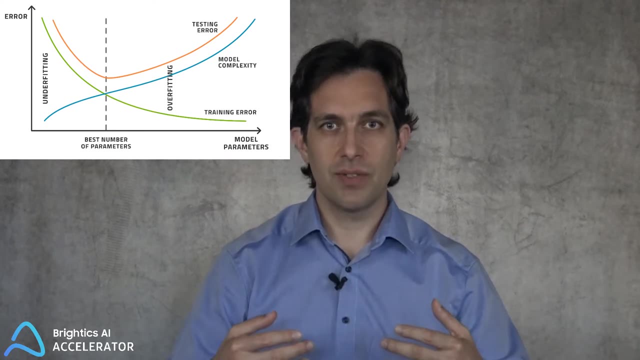 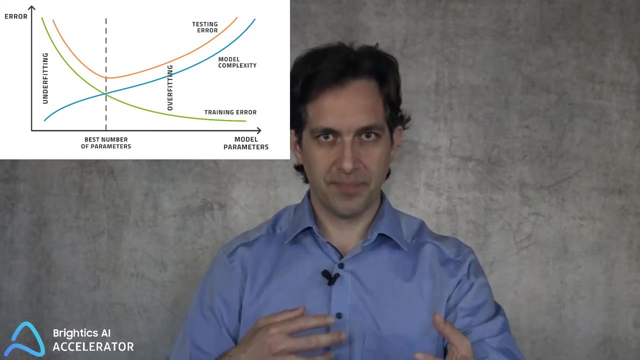 In which case it will overfit. So there is a certain model complexity in the middle of these two extremes which is right Or, if you will, the best. But again there is a trade-off Because clearly, the more complex my model gets. 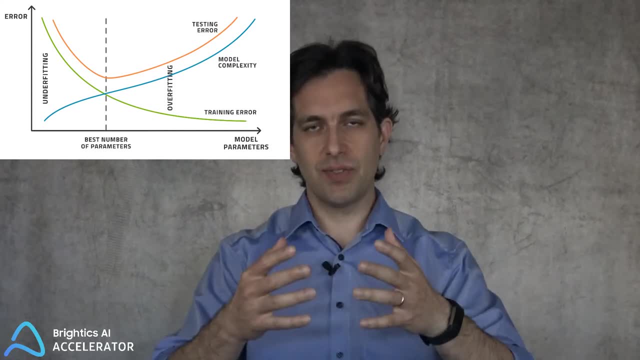 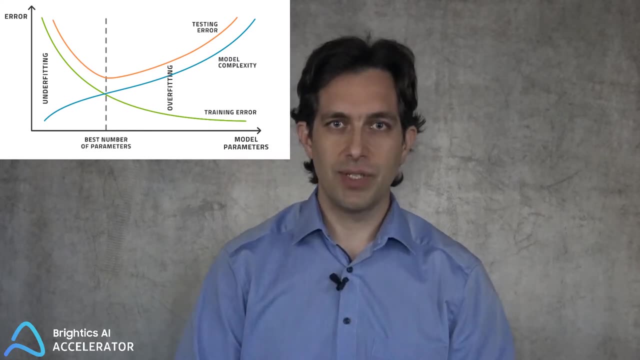 the training error. so the bias over the training data set becomes lower and lower over time. However, the accuracy or the bias over my testing data set- that is, data that the training algorithm does not see- that first of all goes down and later on rises again. 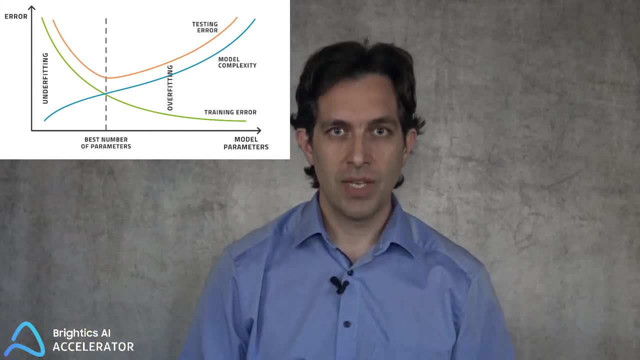 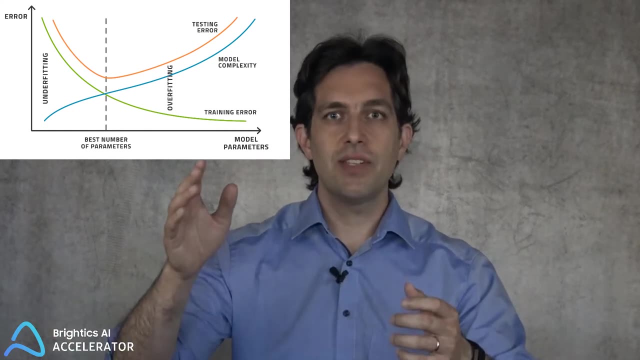 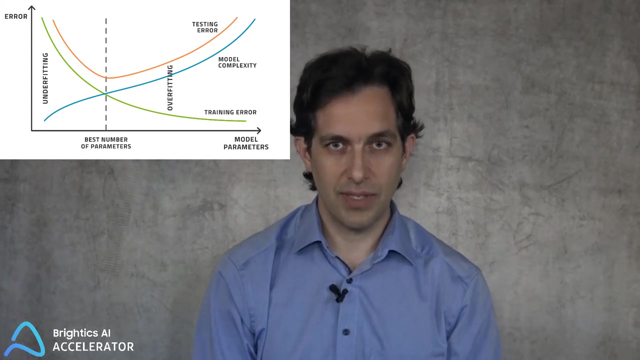 As model complexity increases. So that's my first hint, right As I see model complexity increasing, the testing error first goes down and then goes up. So that's a way to determine the right model complexity. So this is partly an answer to model selection. 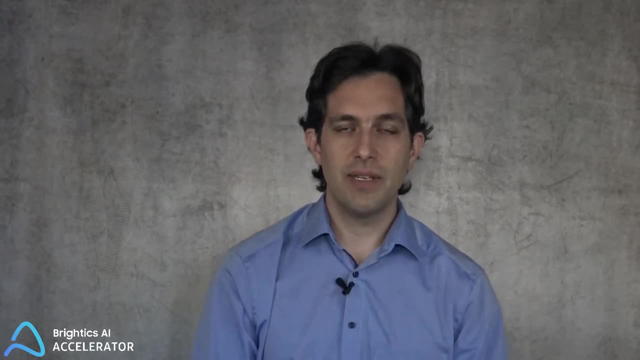 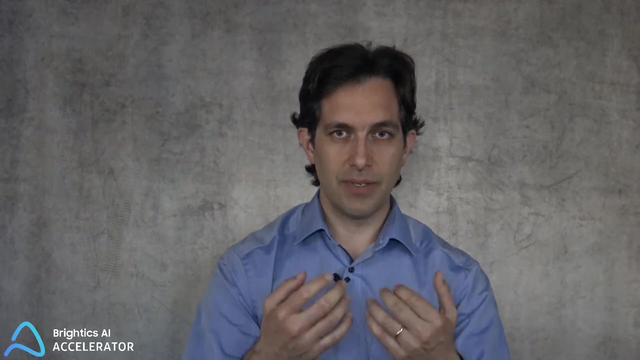 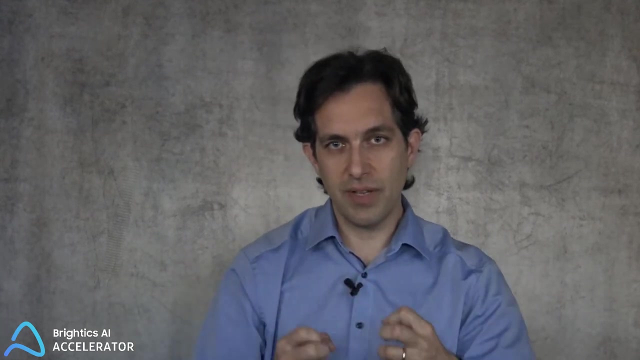 We approach it in this fashion. The variance and bias is, however, a trade-off right. The more I want to gain in lowering my bias- actually, experience shows us that the variance goes up- The more I want to lower the variance. 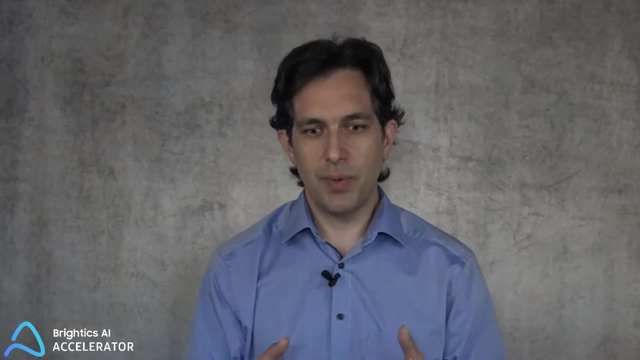 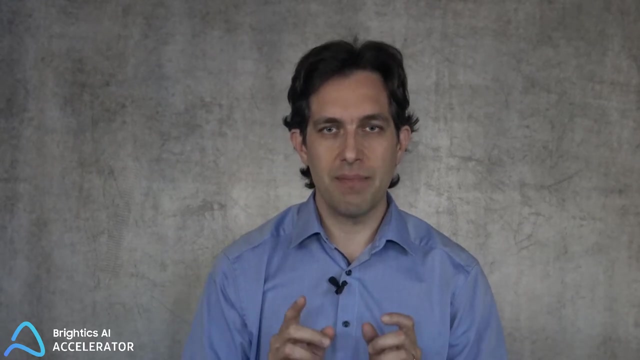 the higher the bias gets. So at some point I need to make a trade-off between these two things. And this is where it comes down to the important question: how do I measure better? Do I measure it in the least squared sense? 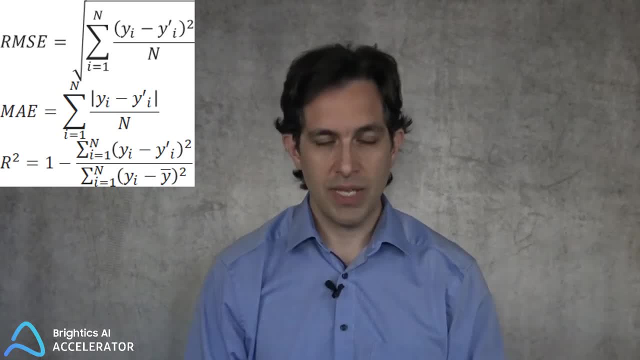 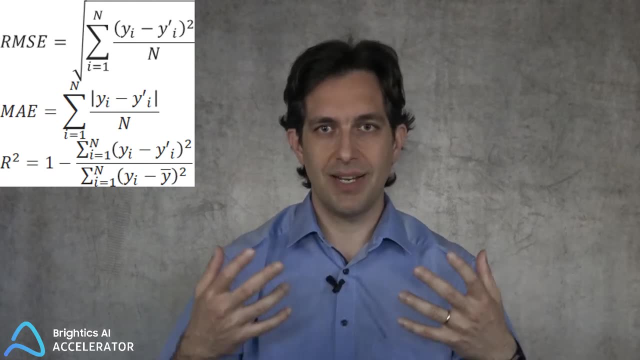 where I add up the residuals and take the square root. Do I measure the mean absolute error? Do I measure the root mean square error? Do I measure some other kind of error measure by which I compare these two By defining the error measure that you use? 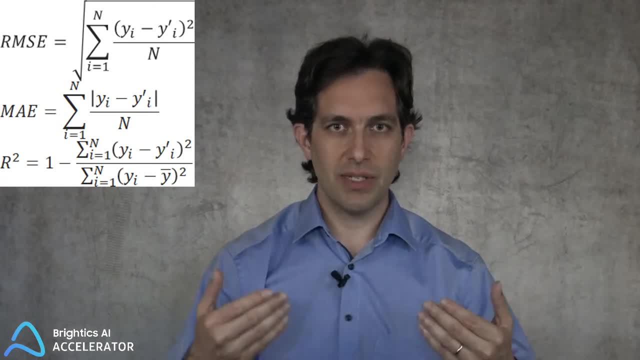 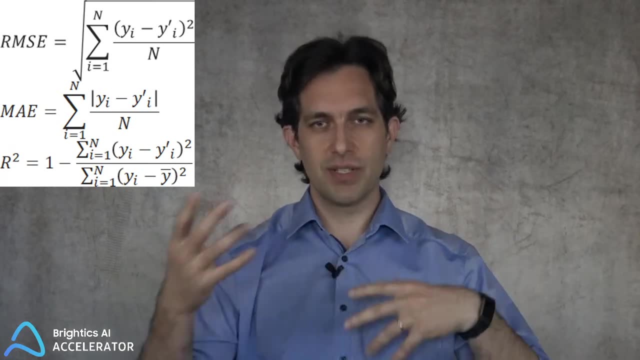 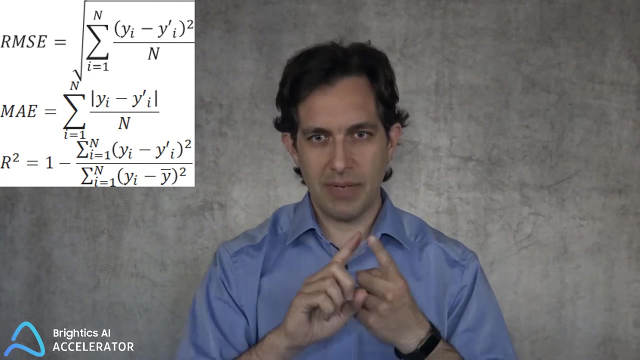 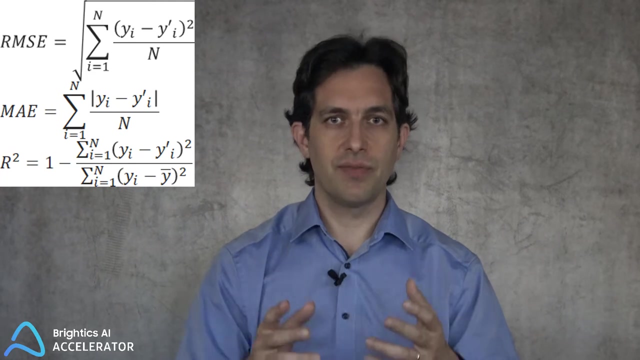 to compare two possibilities, you are implicitly defining whether you prefer variance or bias, or model complexity or some combination thereof. So be aware that when you ask the question, what is my best model, What is the best hyperparameter setting, You first have to define. 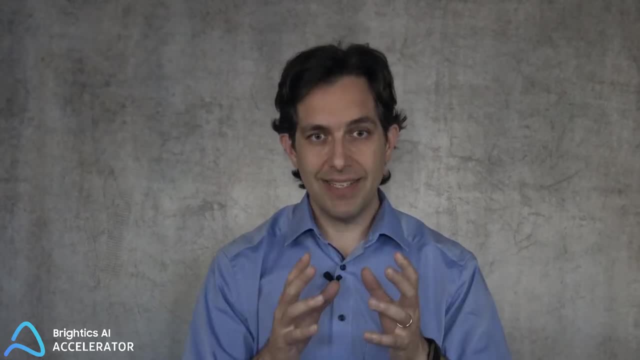 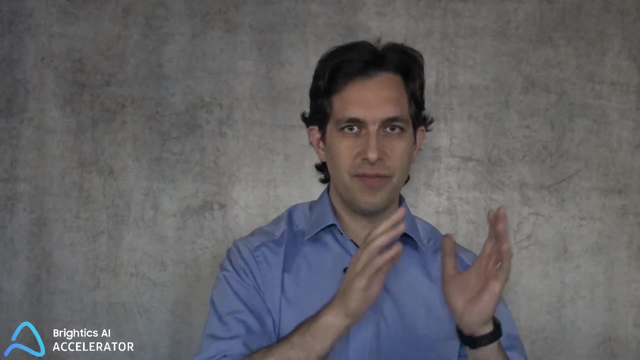 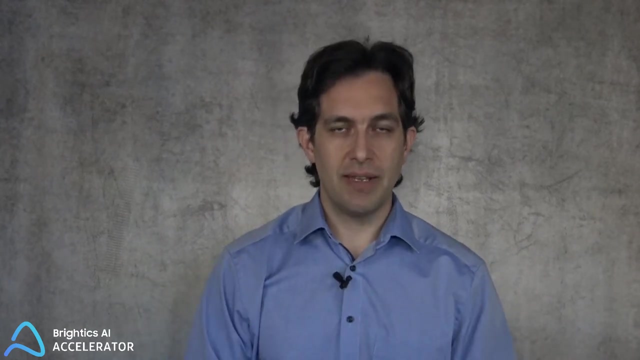 what you mean by best or better. Having done that, you can now train your model on various model topologies with various hyperparameter settings and pick the best one. Typically we would do that manually. That means we would choose maybe three, four, five. 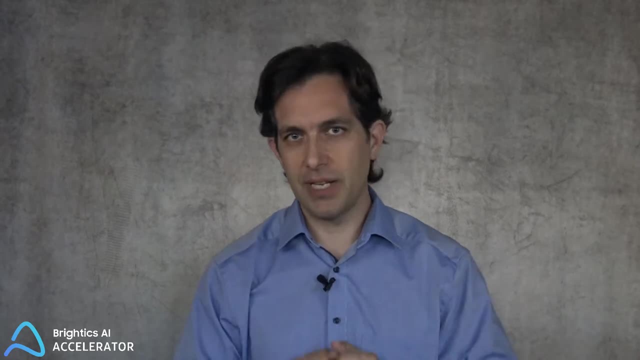 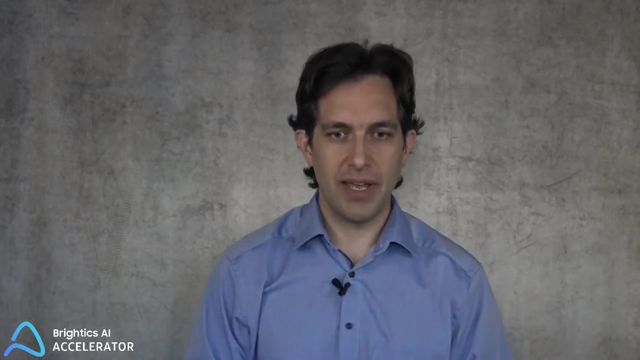 different model topologies. We might choose three, four, five different hyperparameter settings and try them all out, And after we've done all that we kind of manually look over it, mull it over and choose the best one and that's it. 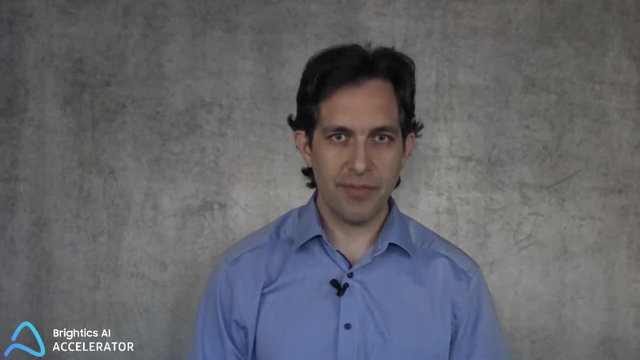 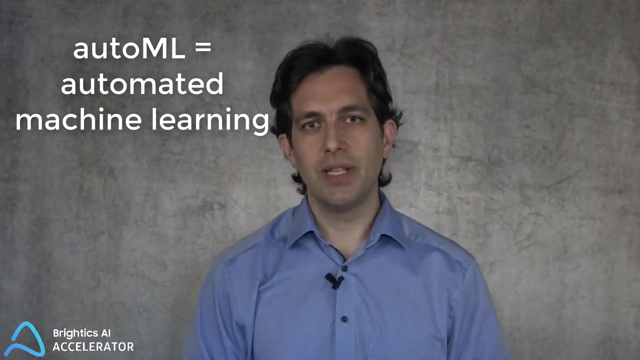 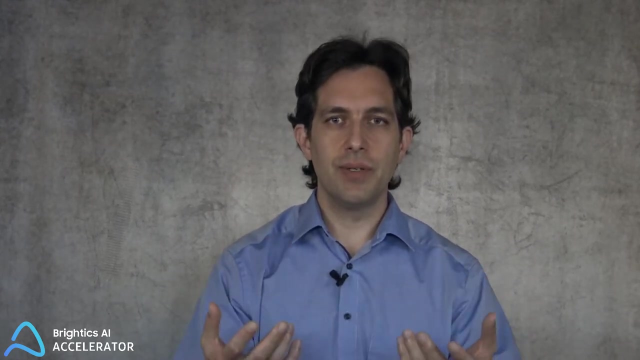 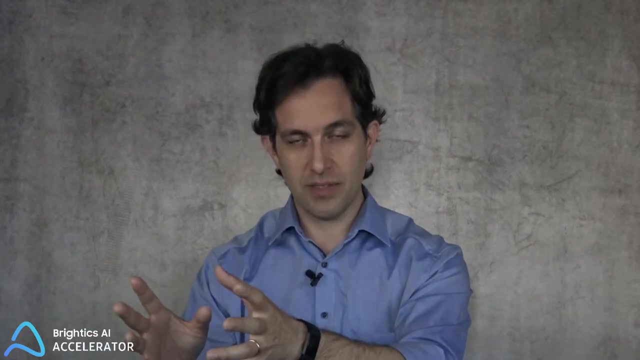 That's some work. It requires time and effort. You can automate this. This is called auto machine learning, auto ML, And that will execute these various experiments for you automatically and give you the answers. It will then automatically tune itself to search the right part of phase space. 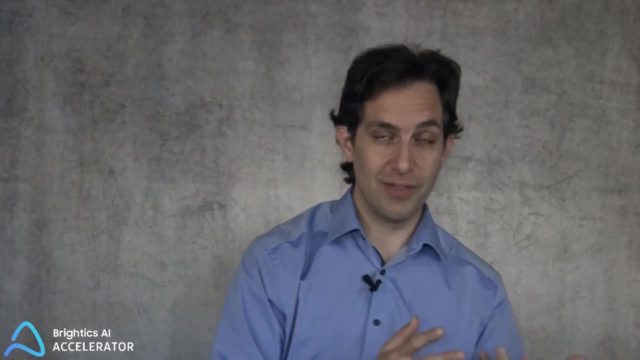 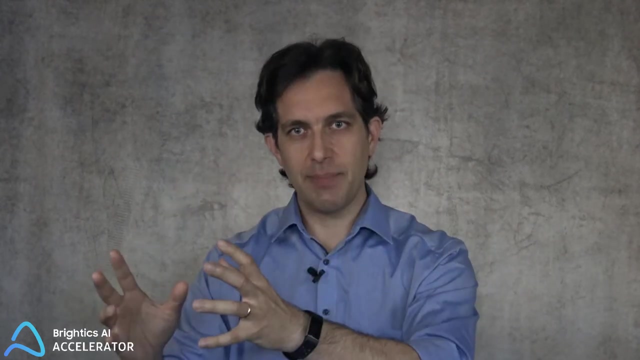 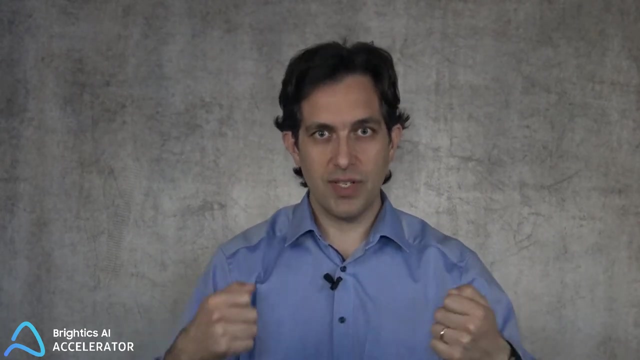 to find the best alternative relative to whatever measure you chose, and present you with the optimal model topology and hyperparameter setting for your model. And in order to do auto ML, the training sequence for a single iteration for a model and hyperparameter setting has to, of course, be fast. 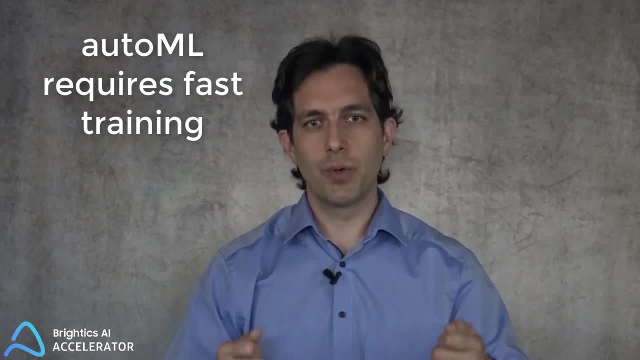 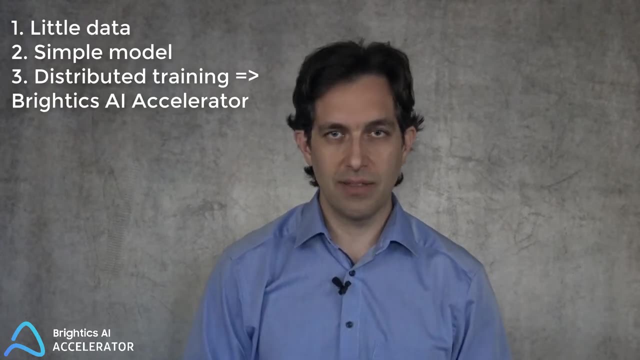 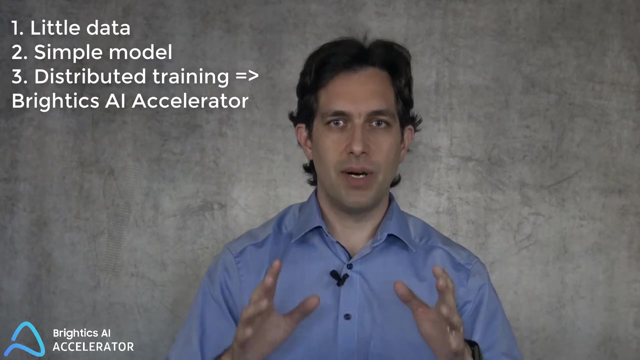 because you have to go through many of these varieties, And in order to improve the speed you need a fast training algorithm. You can accomplish that either if your data is very small or your model is very simple, or by training your model over a distributed cluster of computers.